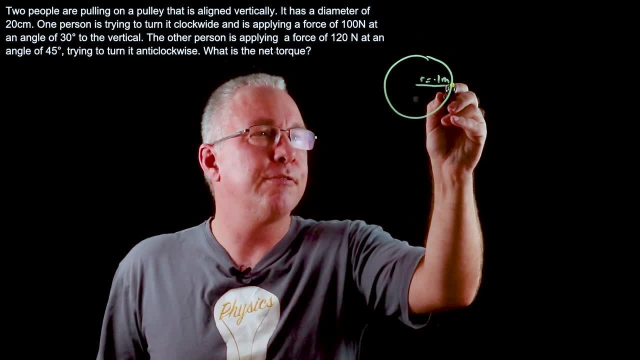 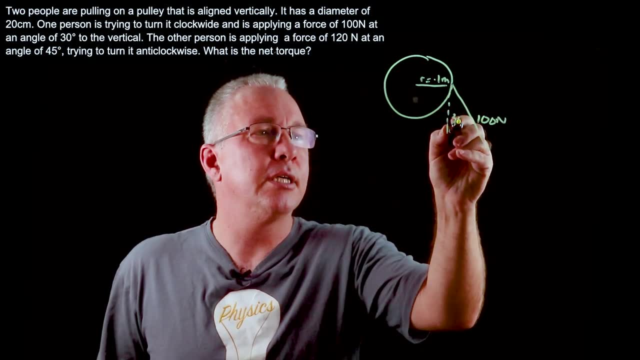 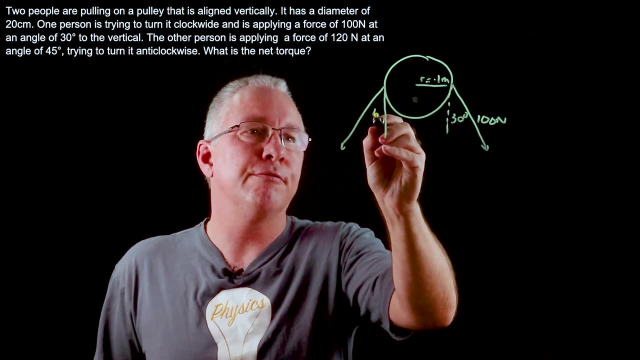 correct SI units. We have two forces being applied. The first force is in this direction, like so, and it's 100 newtons and the angle here is equal to 30 degrees. The other person is applying also a force, in this case at an angle of 45 degrees and it's 120 newtons, and we're asked to work out what is. 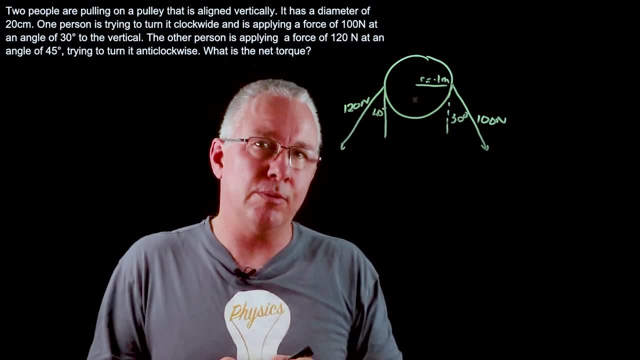 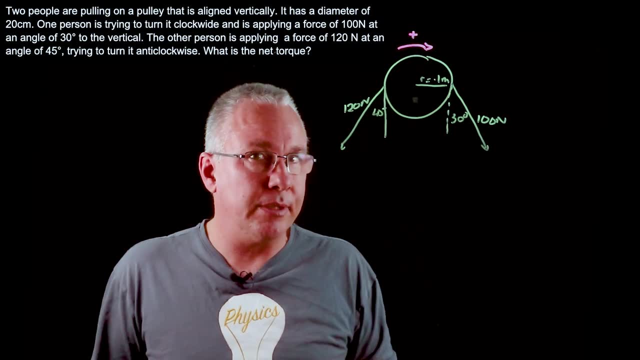 the net torque. Now the first thing you need to do is to determine. what you determine is to be the positive direction. So I'm going to make this my positive direction. I could be wrong. That is, if I work out the net torque and I get a negative value, we know it's going to start to turn the 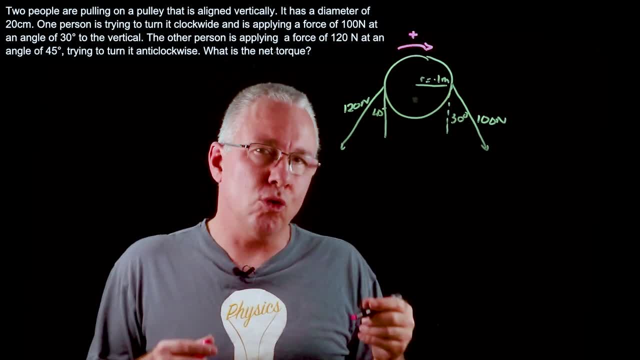 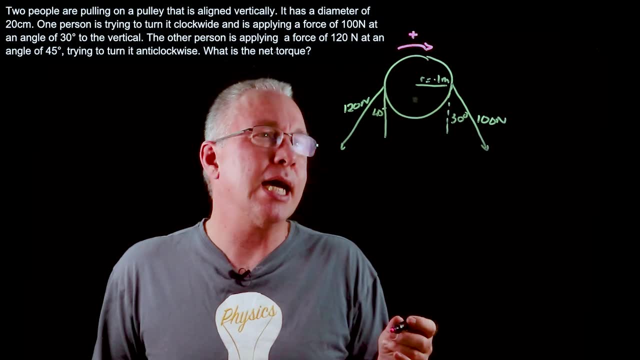 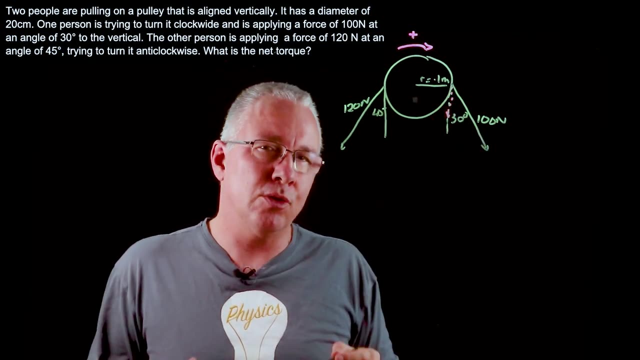 other way. but let's see what happens Now. torque is of course equal to the force multiplied by the perpendicular radius, In other words the moment arm. So, in other words, maximum torque is of course actually acting in this case here, but because this is not actually at that angle, we need to 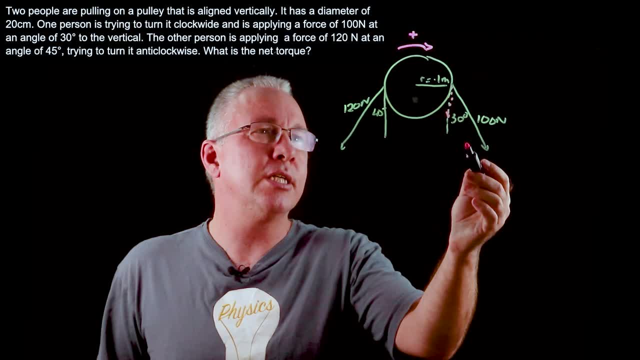 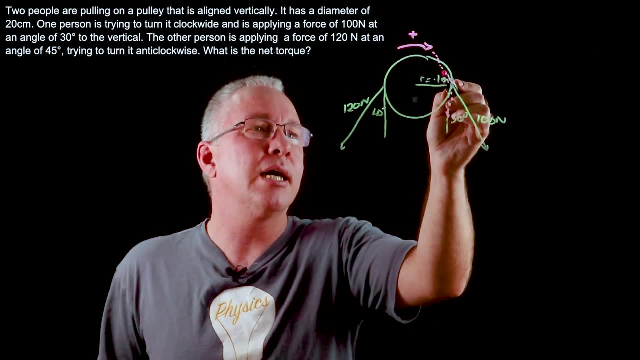 have a component. But what is the component? We know this is 30 degrees, but the angle we're interested in is the angle between that direction and the moment arm, So that it's actually this angle here, That is, that angle between that direction and the moment arm, So that angle. 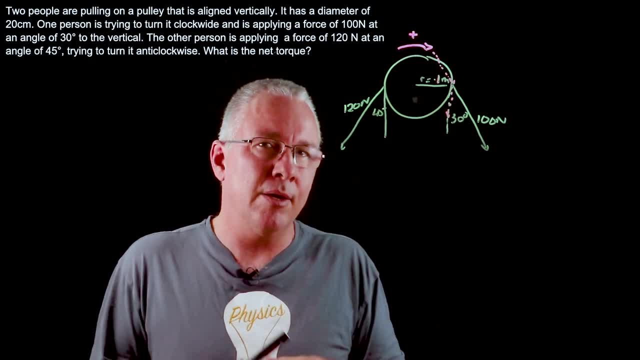 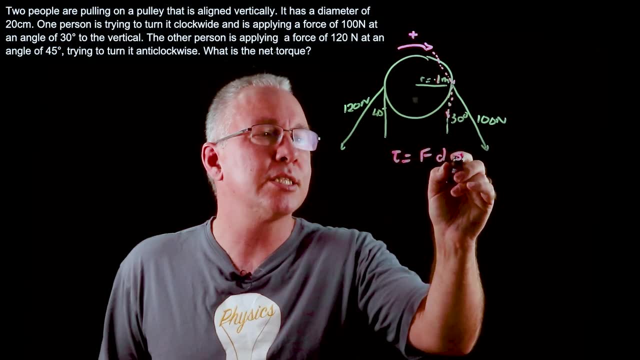 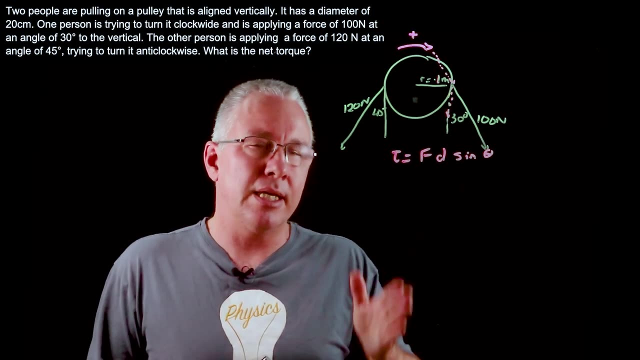 here is going to be, in this case, equal to 60, when we're using the correct formula, because the torque is equal to the force multiplied by the moment r multiplied by the sine of the angle, and the angle is the angle i'm talking about here. it's not 30 degrees, it's 60 degrees. now a way to think about. 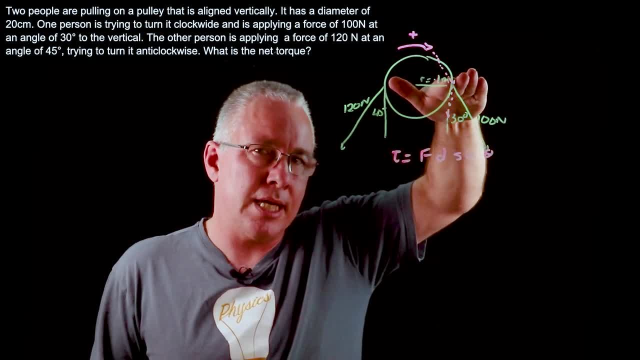 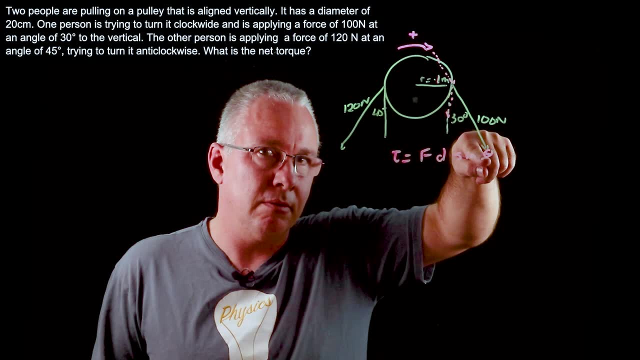 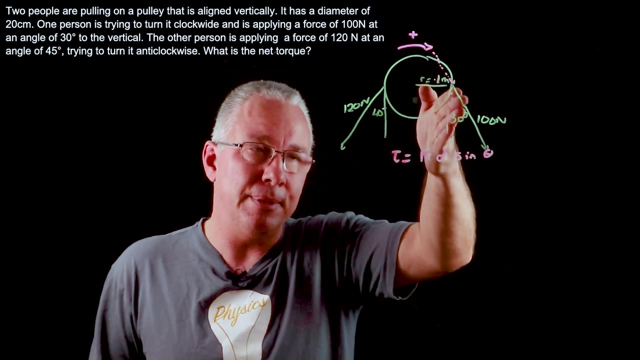 that this is this. if this becomes 90, then as a result, the other angle here is zero, and that means the sine of zero is equal to. well, what is it zero? so we get no torque whatsoever, whereas if it's perpendicular, my angle is actually 90. well, the sine of 90 is one, so we have a maximum torque. so